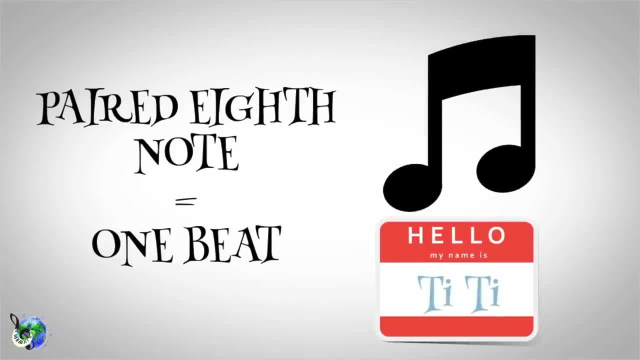 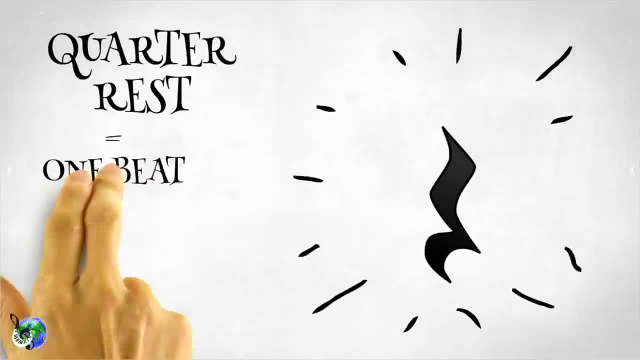 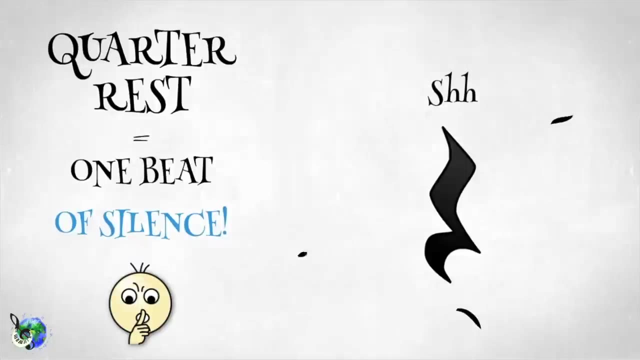 be beamed together, and when beamed together they will equal one beat. We give the paired eighth notes the name ti-ti. Then we have the quarter rest. The quarter rest receives one beat of silence. When we see the quarter rest, you can say shh or simply remain silent. So we So coming. 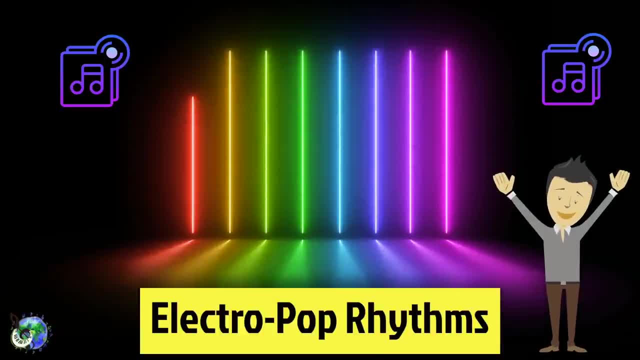 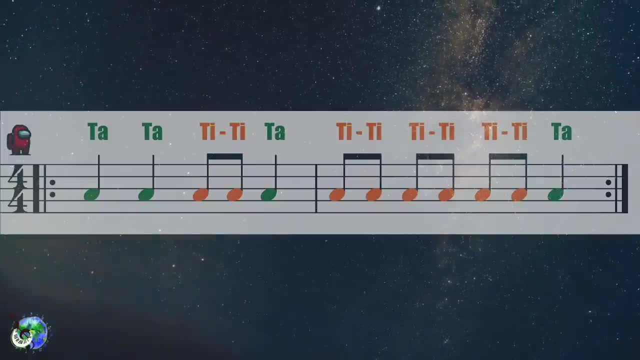 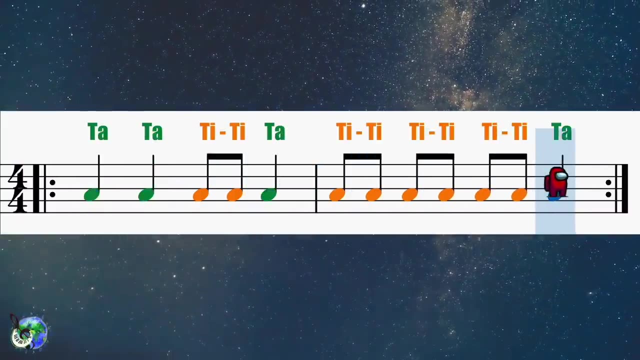 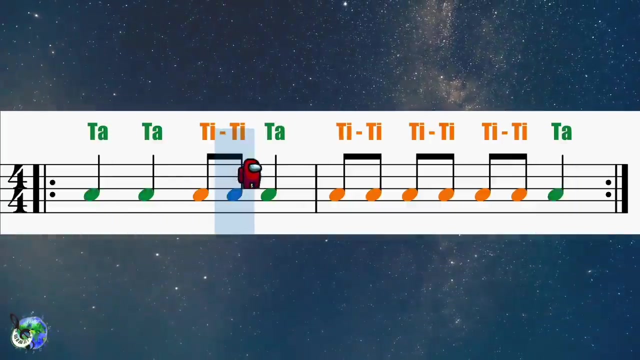 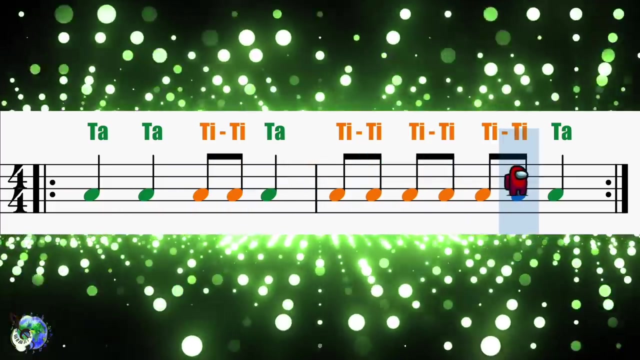 up. you will see rhythms that we will clap along while saying the ta and ti-ti out loud. Oh boy, and look who is among us. Are you ready? One, two ready, go Ta ti-ti, ti-ti, ti-ti ta, Ta, ta, ti-ti ta, ti-ti, ti-ti, ti-ti, ta, Ta, ta, ti-ti ta, ti-ti, ti-ti, ti-ti ta. 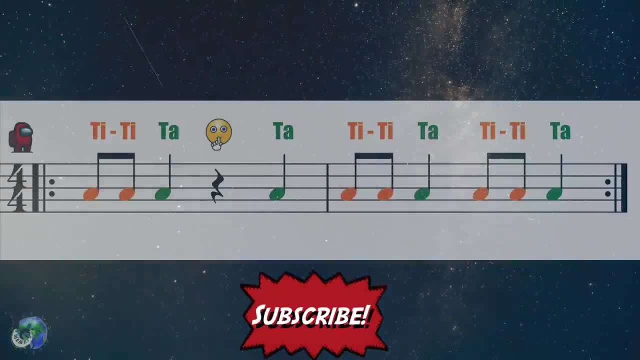 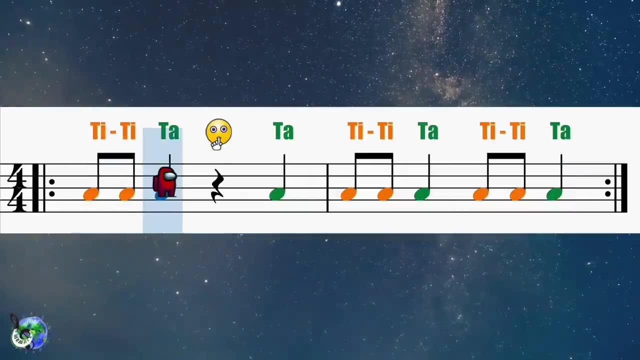 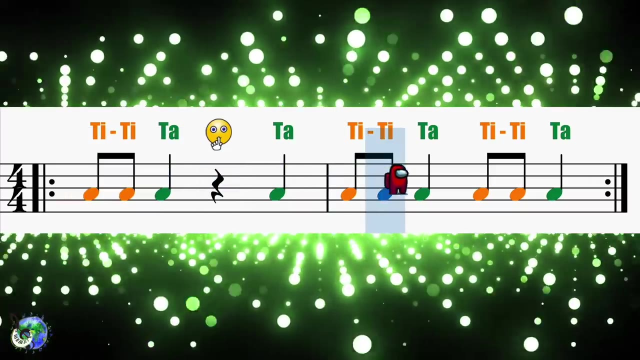 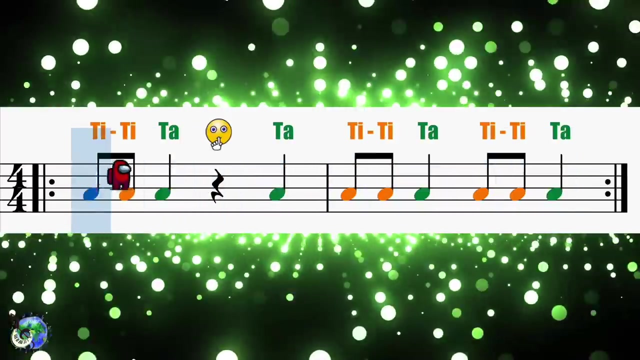 Awesome, Let's get ready for the next rhythm. Take a look and a quick study. One, two ready, go Ti-ti ta ta, ti-ti ta Ta, ti-ti ta, ti-ti ta Ta ta, ti-ti ta, ti-ti ta. 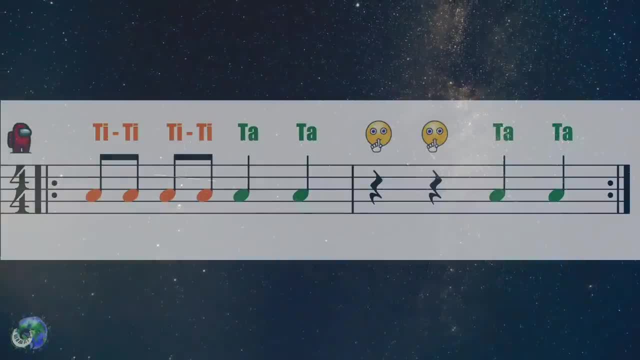 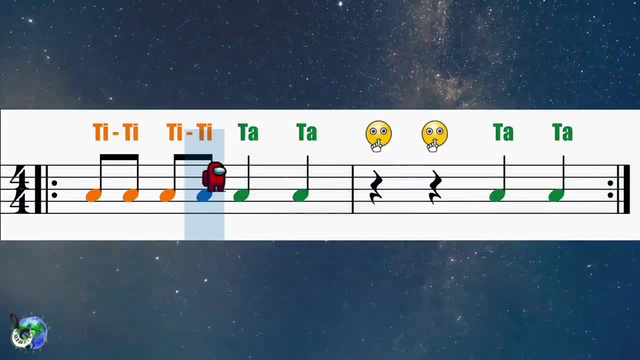 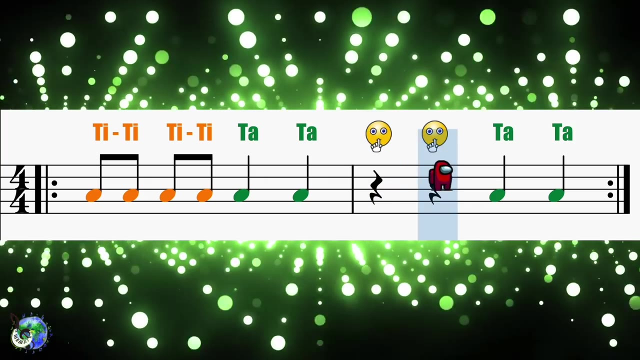 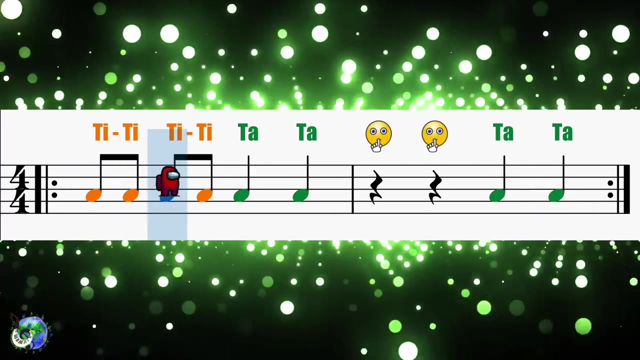 Super cool. Let's get ready for the next rhythm. This time you are on your own. One, two ready. go Ti-ti ta, ti-ti, ti-ti, ti-ti sta, Ti-ti ta, ti-ti ta ti-ti-ti. stop, si, si, si. 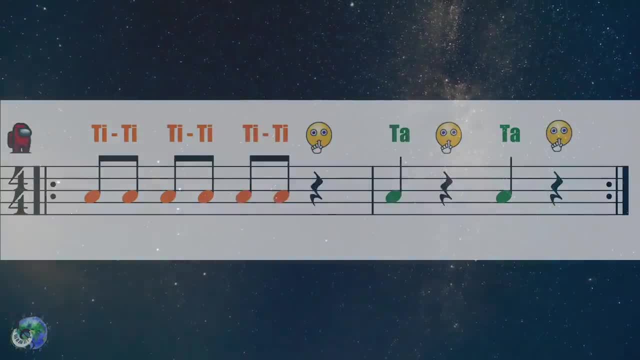 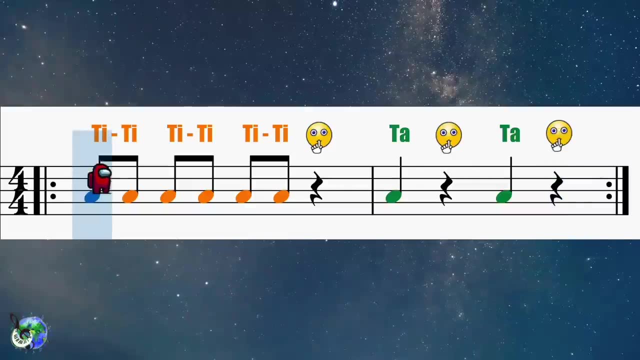 Ti-ti ta, ti-ti, ti-ti. Excellent, Let's get ready for the next rhythm. Take a look and a quick study. One, two ready. go Ti-ti ta, ti-ti, ti-ti, ti-ti, ta-li, stop si si, temi-ni si si. Ti-ti ta ti-ti ti-ti ti-ti stop si si si si Ti-ti ta ti-ti ti-ti ti-ti ta Ma mi mi ti-ti ma ti-ti ta topき siin Ci. 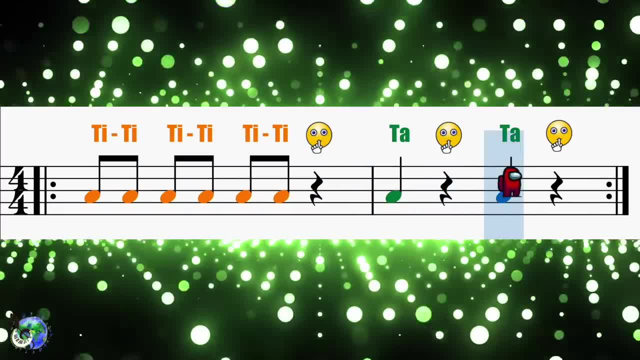 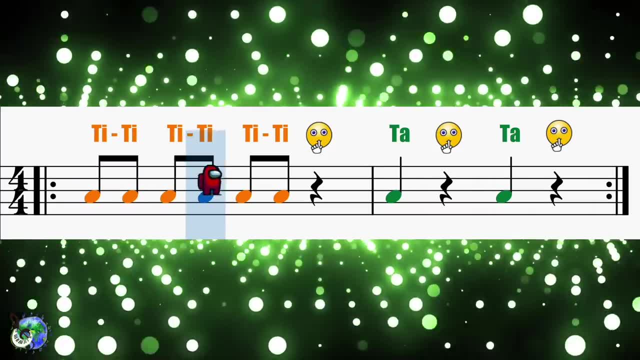 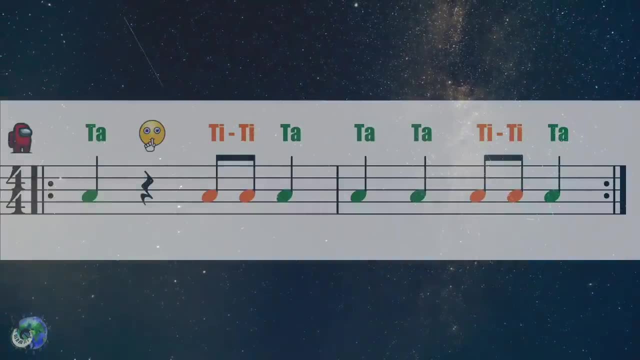 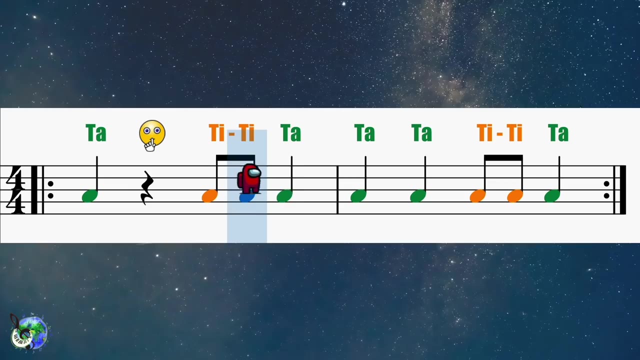 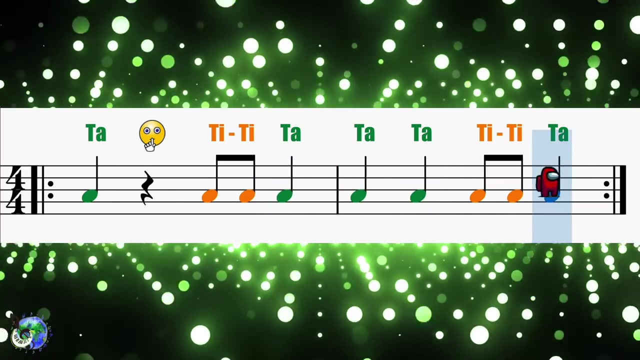 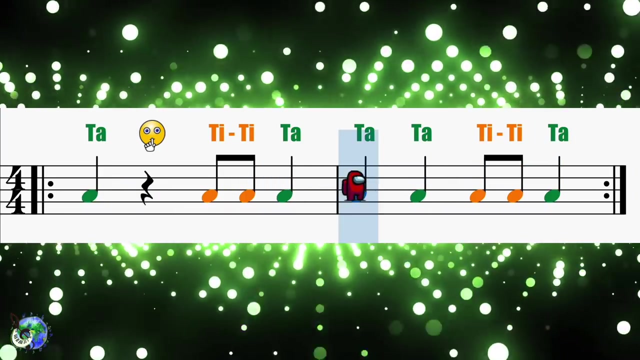 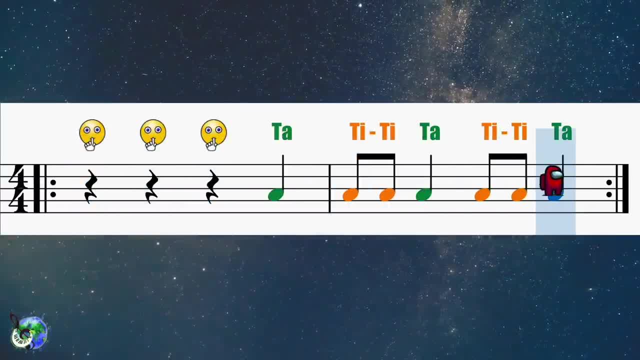 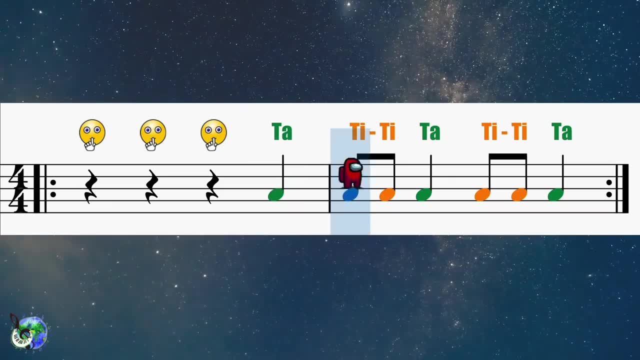 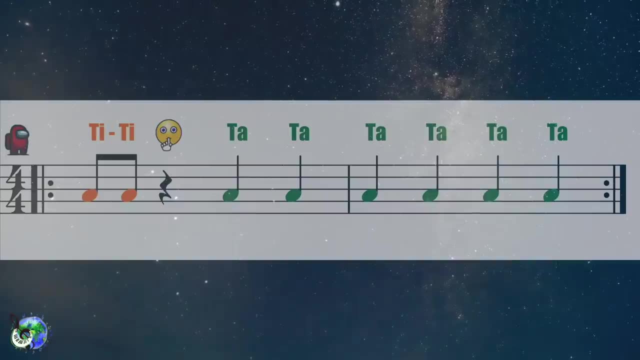 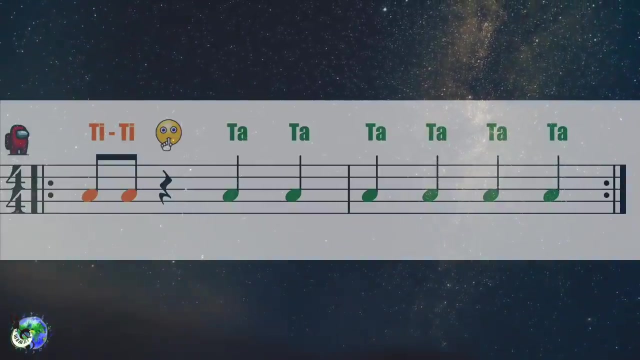